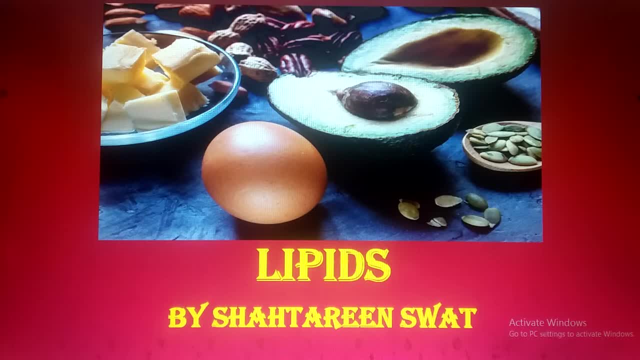 and in this lecture I will discuss about the introduction and what are basically the lipids are, and classification, and I will discuss in detail about the first, simplest lipids, which are known as triglycerides. So keep watching, keep sharing knowledge with others, like my videos. 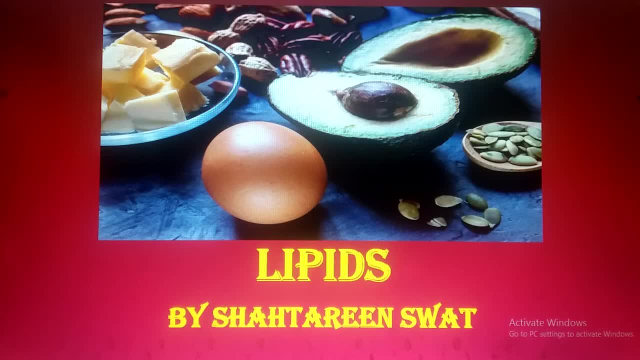 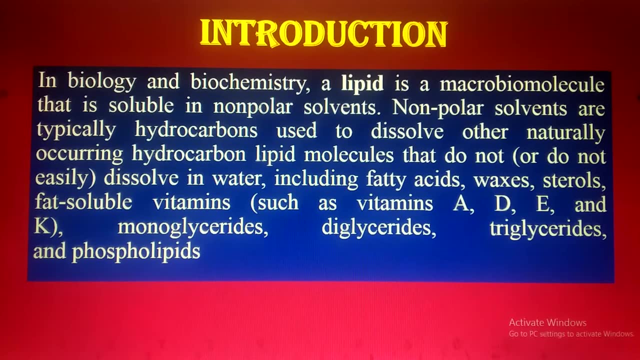 share my video, subscribe to my channel and promote my channel. Now I am going to start, and first of all, what are basically the lipids? In biology and biochemistry, a lipid is a macromolecule that is soluble in non-polar solvents. Non-polar solvents are typically 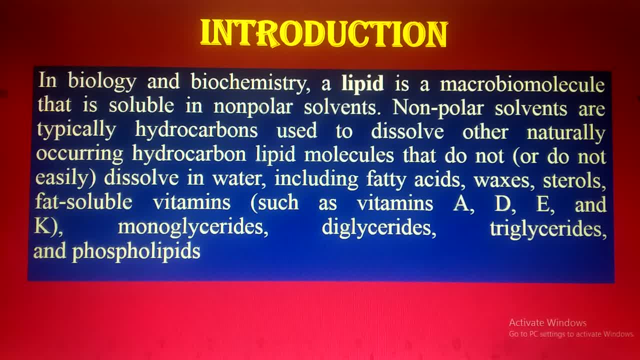 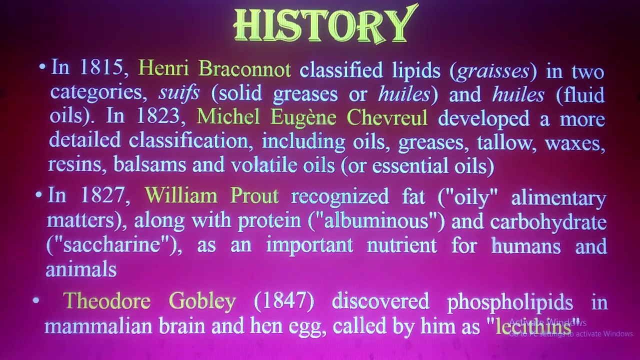 hydrocarbon used to dissolve other naturally occurring hydrocarbon lipids molecules and do not dissolve in water, including fatty acids, waxes, steroid fat soluble vitamins like vitamin A, D, E and K. Now I have a little bit about the history of the lipids. There are a diverse group of 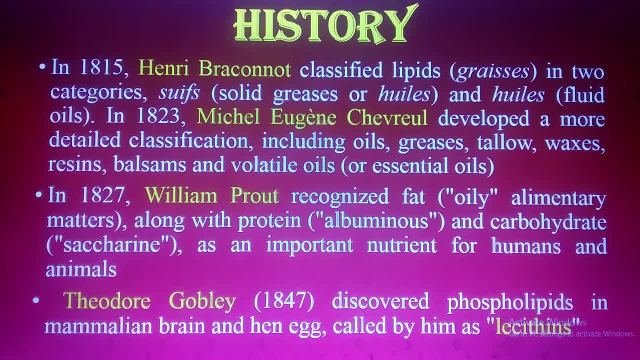 the scientists who worked on lipids, and I have some information for you. In 1815, Henry Briquenez disclassified lipids in two categories: do you feel? and you You feel? these are the French words, so you can pronounce as you can. So your face, our solid grease and wheels is 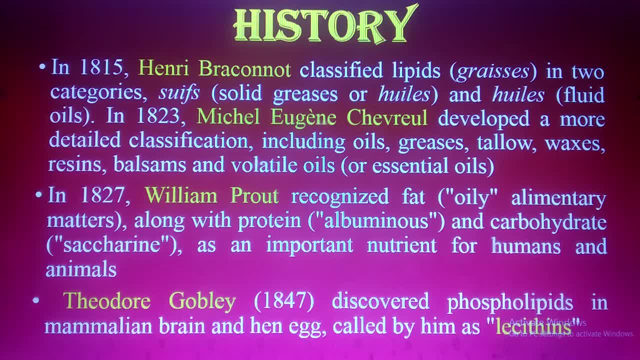 a fluid oil. In 1823, Michel Eugène developed a more detailed classification including oil, grease is solche, vacas, raisins and volatile oil. in 1827, william prout recognized fat, oily elementary matter, along with protein, albuminase and carbohydrate saccharin. i have discussed proteins and carbohydrates in. 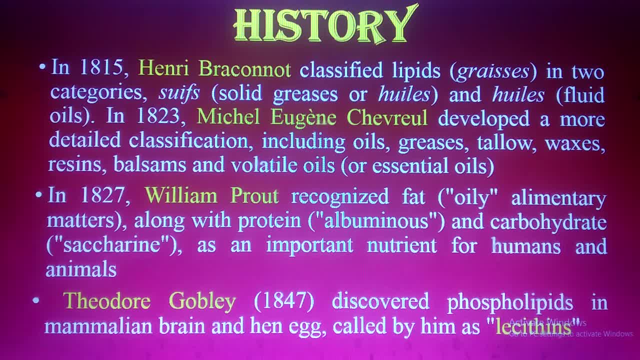 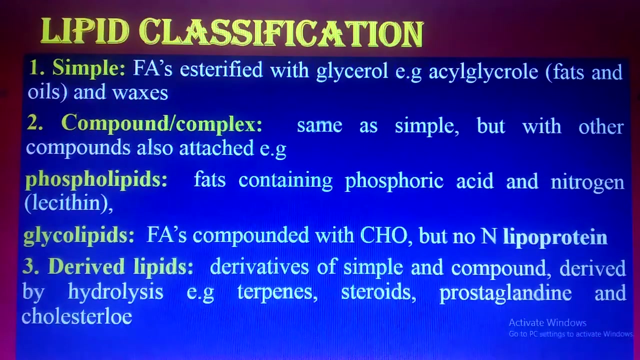 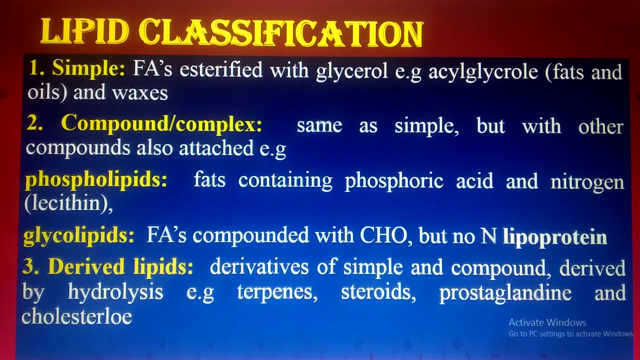 detail, so must go through my lectures about the proteins and carbohydrate as an important nutrient for humans and animals. then theodore gobley in 1847 discovered phospholipids in mammalian brain and hen egg, called by him as a lacy thin. okay, now the classes. there are major three classes are: categories of the lipids: simple lipids, compounds. 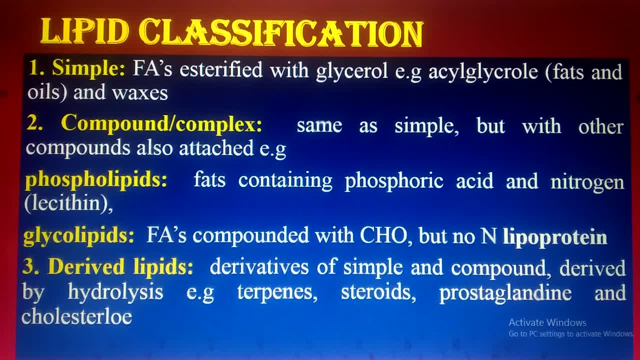 are complex lipids and the derived lipids. so for say, simple lipids are produced by the action of the or by the reaction of the fatty acids with glycerol, and the reaction is known as, the reaction type is known as acidification. so fatty acid, what are fatty acids? fatty acids are basically the building units of the lipids, like amino acids. 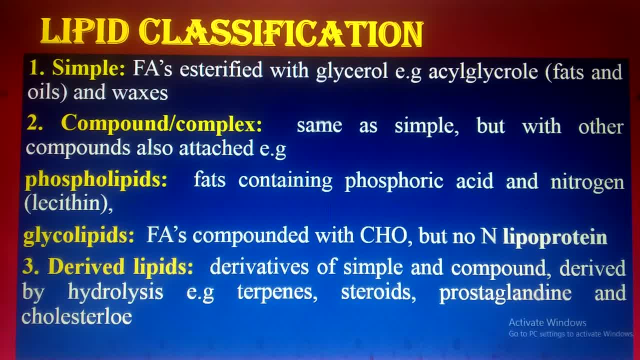 are the building units of the uh. proteins and monosaccharides are the building units of the carbohydrates. similarly, fatty acids are the building units- or you can say that the building blocks- of the uh lipids, fats. so fatty acid estrophied with glycerol produces the simple lipids compound. 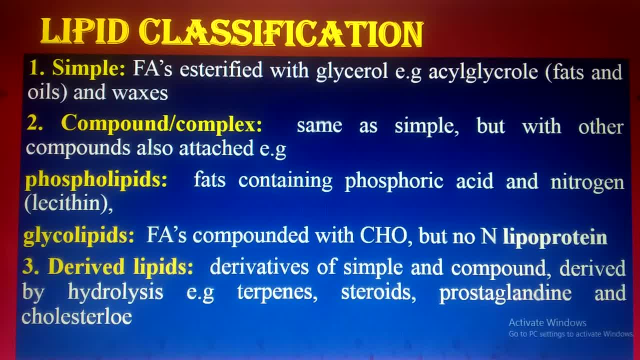 are complex, same as simple, but with other compounds also attached, for example phospholipids, glycol lipids and the derived lipids. third one, derived lipid lipids. as the name indicated, derivative lipids also call as hyaluronic acid, also known as glycol lipids, inteligular lipids, tolls Sukogli lipide is commonly used in the use of polycy. 갑gii lipid lipid lipids. areoston free lipid lipid lipids with glycoglipid lipids are so bağish thatosse cucumber lipids create source of fathers lipid lipids. traditional lipids is not considered surgery lipid or lipid 거의 lipides in place of underlipped lipids. 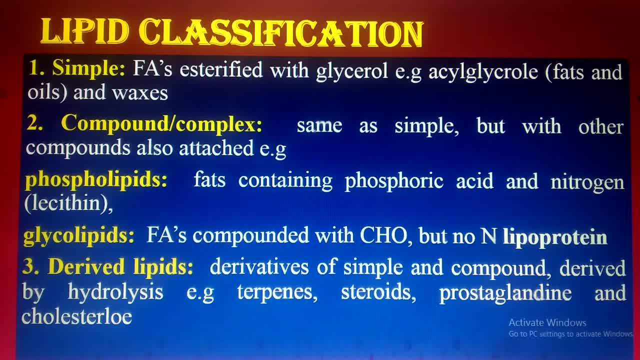 one derived lipids, as the name indicated, derivatives of the simple and compounds derived by hydrolysis, for example, hydrolysis of the simple and compound lipids like terpenes, steroid prostaglandins and cholesterol. okay, now the biological role. i will discuss all the 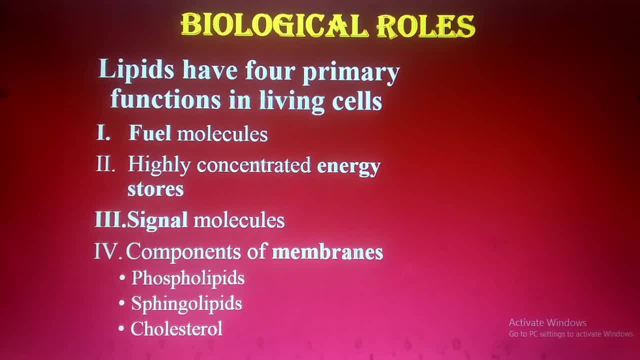 lipids and their all different types of the lipids and their role in the human life and other plants and also in the animal. so uh biological role in as a fuel they are used uh high energy stored molecule, signal molecule. they are also used help in the cell signaling uh and the component. 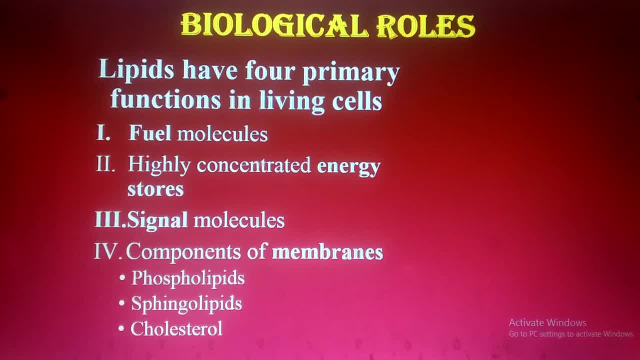 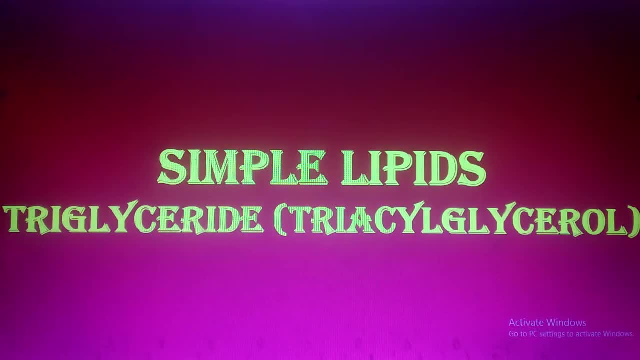 very important: the component of the membranes in the form of the fossil lipids, sphingolipids and cholesterol. first of all, i'm going to uh discuss in detail about the cell lipids and their role in the human life and also in the animal. so biological role as a fuel. 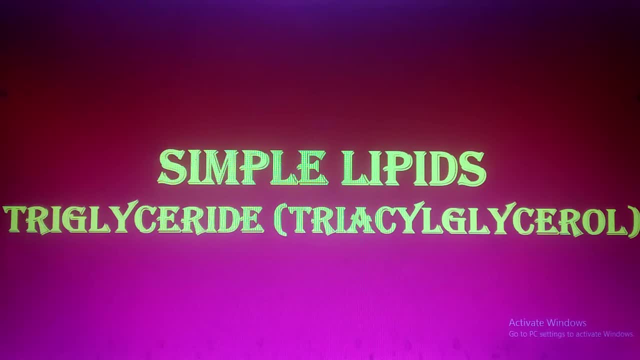 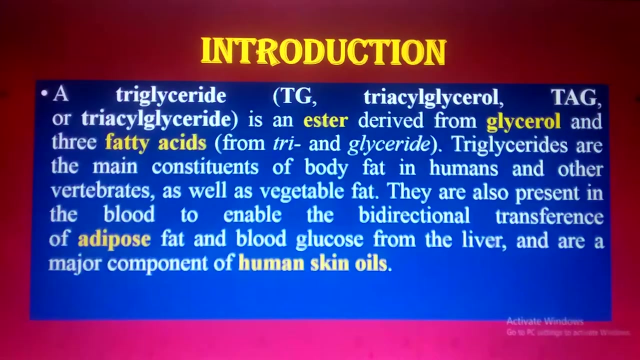 type of the lipids which are simply um produced uh by the reaction uh, which is known as esterification of fatty acids, and glycerol. they are called triglycide or triacylglycerol. why they are called triglycide? the reason is that the they are made up of the three fatty acids. 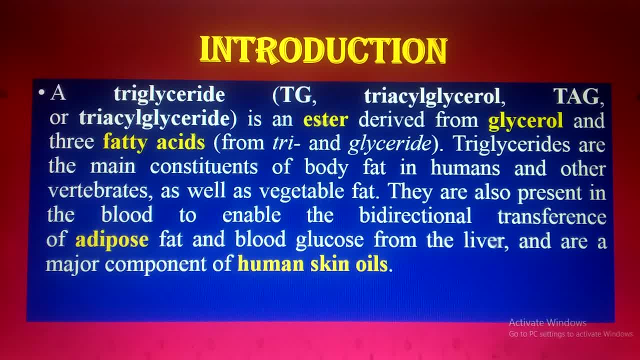 with one glycerol. glycerol is an alcohol and three fatty acids. that's why this is known as triglyceride. triglycerides are the main constituents of the body fats in humans and other vertebrates, as well as vegetable fats. they are also present in the blood to enable the 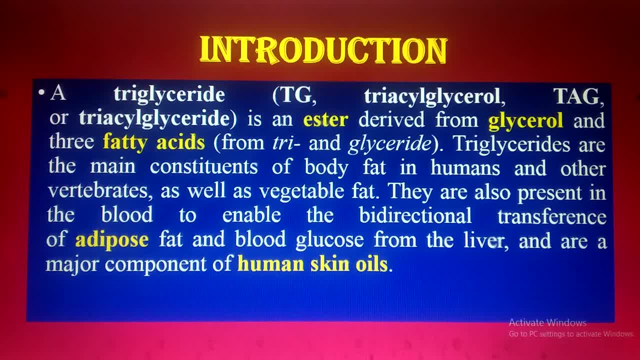 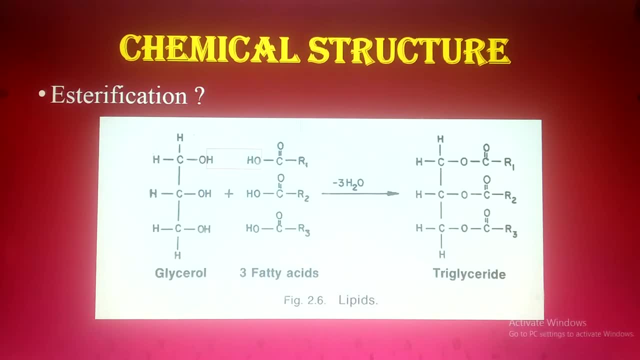 biodegradable transference of the adipose fats and blood glucose from the liver and are a major component of the human skin's oil. okay, now this is the chemical structure of the triglyceride, and you can see here the chemical reaction which is known as esterification. uh, in esterification, one glycerol react with the 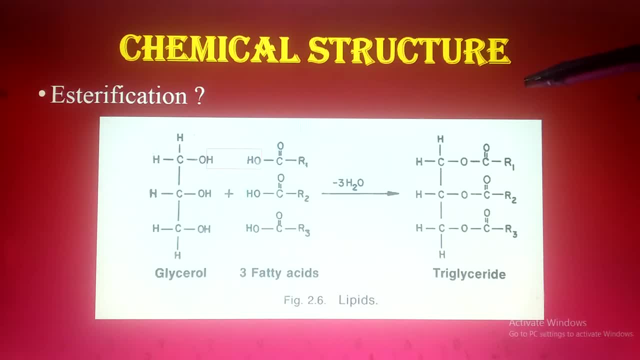 three fatty acids. and during esterification what will happen? uh, hydrogen ion is removed from the glycerol, alcohol and hydroxyl ion is removed from the fatty acids. so one hydrogen from the glycerol and oh group from the fatty acids produces the water molecules. so you can see. 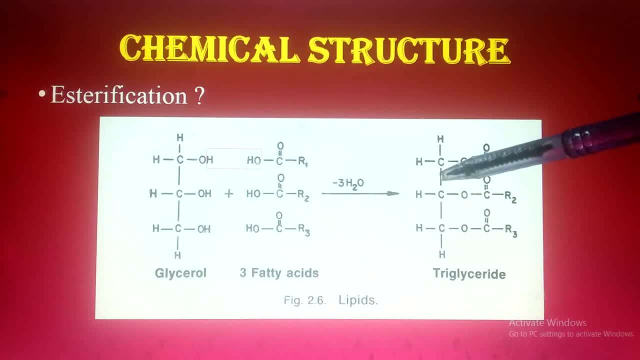 three water molecules are produced because three fatty acids are present: uh and uh. three uh carbon atoms are present: the glycerol. the glycerol is a three uh carbon containing uh alcohol. so you can see here the esterification mechanism in which three fatty acids react with the glycerol and produces the triglyceride. 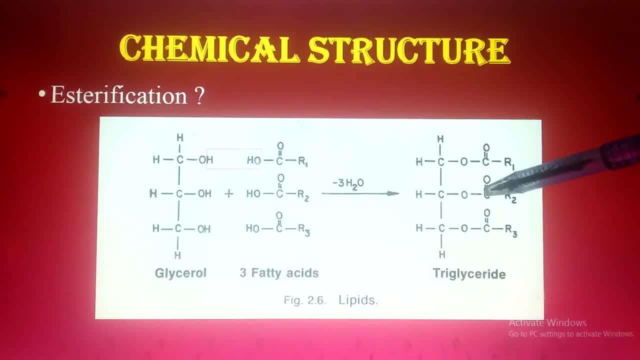 so this is the simplest uh structure of the triglyceride, or chemical structure of the triglyceride. and what is esterification, in which a hydrogen ion removed from the glycerol and the fatty is uh, hydroxyl ion removed from the fatty acids and the bond is produced? 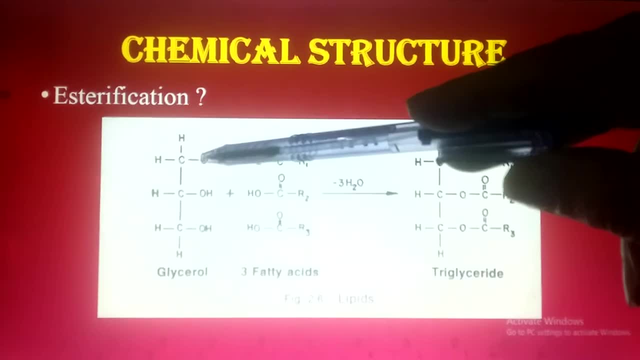 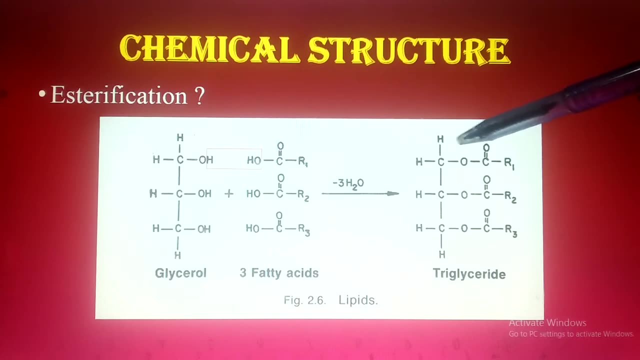 between the uh oxygen of the uh glycerol with the carbon of the fatty acids. so this is uh- by the removal of the water molecule. so this is the simplest mechanism of esterification in which triglycerides are produced. is it clear? okay, now classifier. 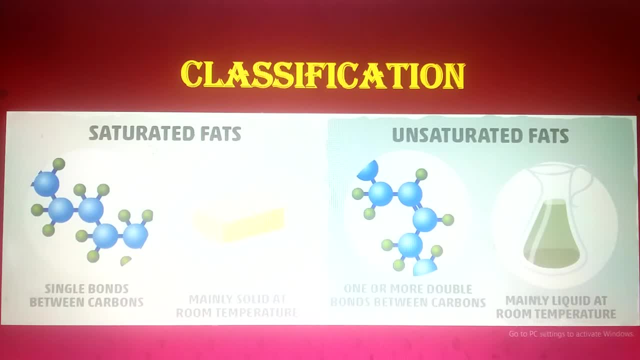 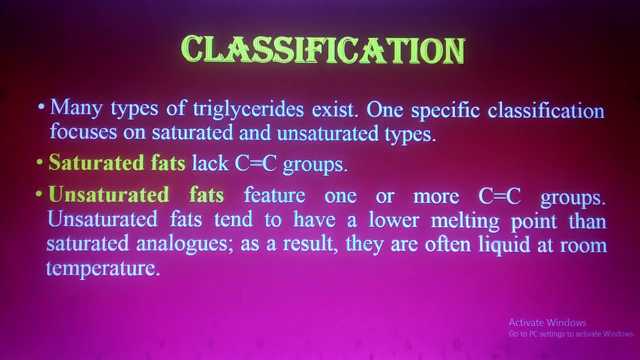 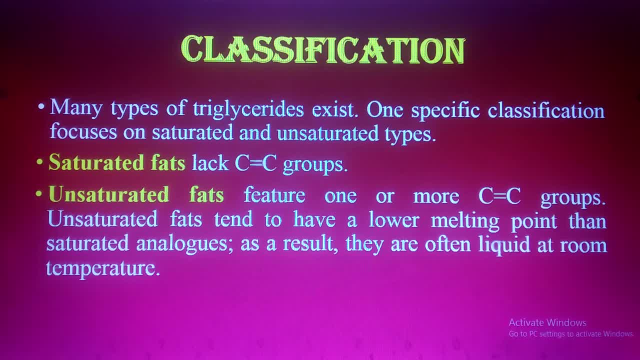 and in unsaturated fatty acids one or more double bond present. unsaturated fats tend to have a lowest lower melting point than the saturated analogs. as a result they are often liquid at room temperature. so the concept clear about the saturated: saturated they lake the bond, double bond, and unsaturated they have double bond. so saturated fats consist of the. 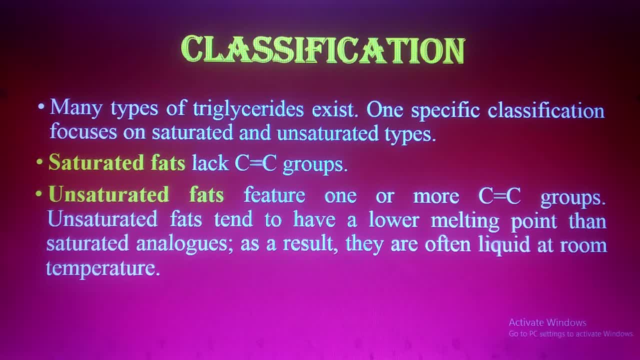 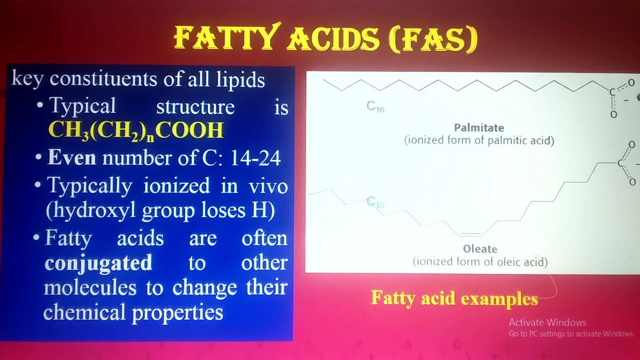 saturated fatty acids. they are solid at room temperature and unsaturated are, have low melting melting points and have double bonds and one or more than and they are liquid at room temperature. saturated are solid and unsaturated are liquid. so fatty acids, which is you can say, which are the building units, are building blocks of the 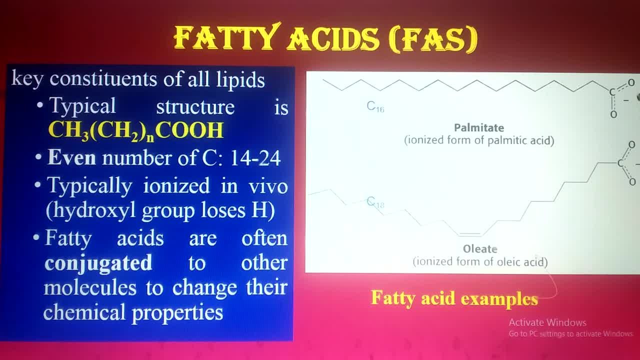 fats are lipids, typically the structure you can see here: ch3, ch2, cooh. even number of carbon 14 to 24 carbon. even number of carbon 14 to 24. carbon 14. fatty acids consist of 14 to 24 carbon atoms, typically ionized in vivo hydroxyl group. 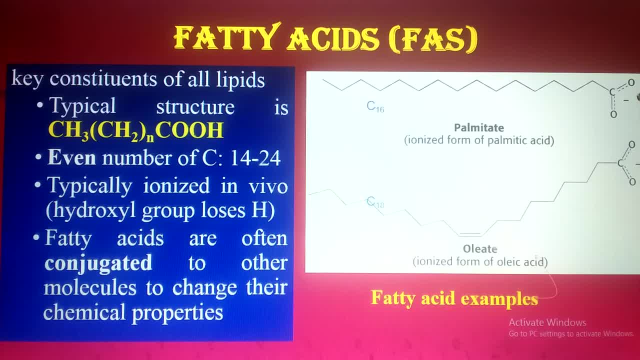 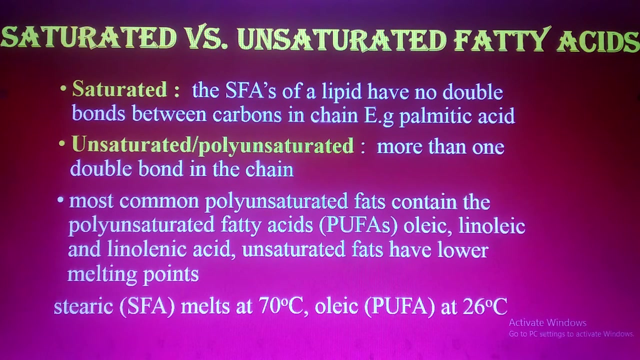 loses hydrogen. fatty acids are often conjugated to other molecule to change their chemical properties, like with sugar, molecules like proteins, amino acids and many more. so the key constituents of all the lipid is fatty acid. now, two types of the fatty acids exist: saturated fatty acids, as i have discussed. uh, having uh. 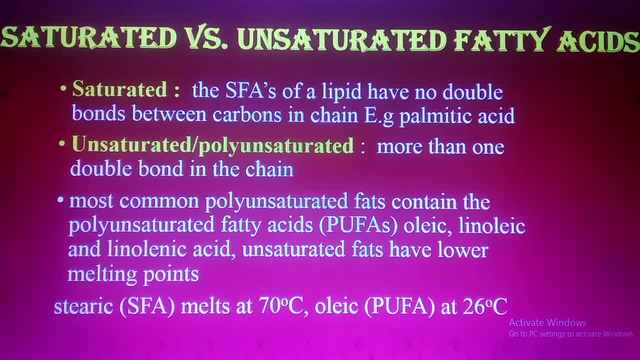 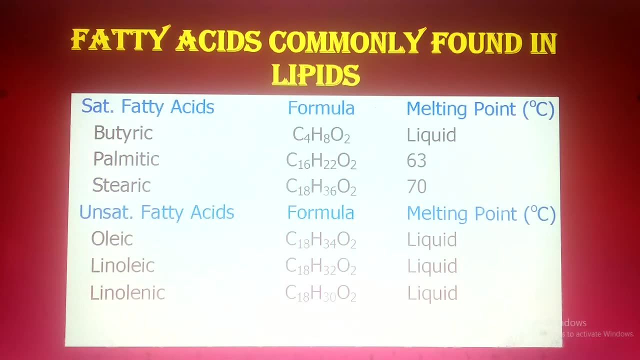 no, uh, double bond and the unsaturated acids, they have uh double bond, more than one double bond in the chain and there are- i have some exam examples of the saturated and unsaturated fatty acids for you people. so you can see here, uh, the saturated fatty acids, uh with. 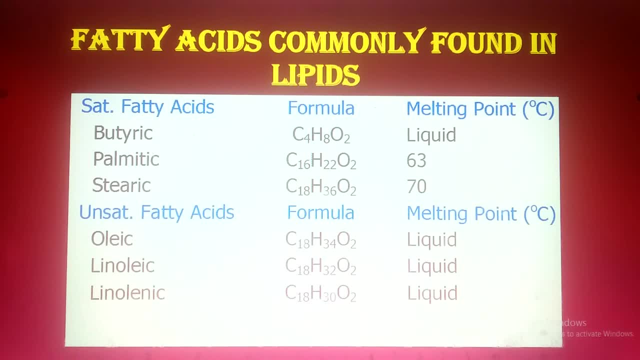 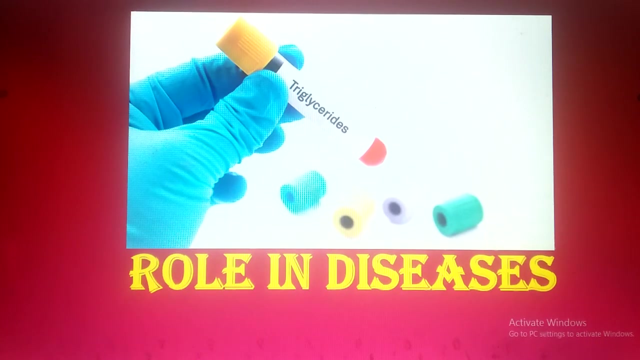 their chemical formula and melting points: butyric, palmitic, uh, stearic. they are the saturated fatty acid, unsaturated oleic, linoleic and linoleic acids. these are the unsaturated and these are the saturated. okay, first let's talk about the role of the triglycerides in diseases. 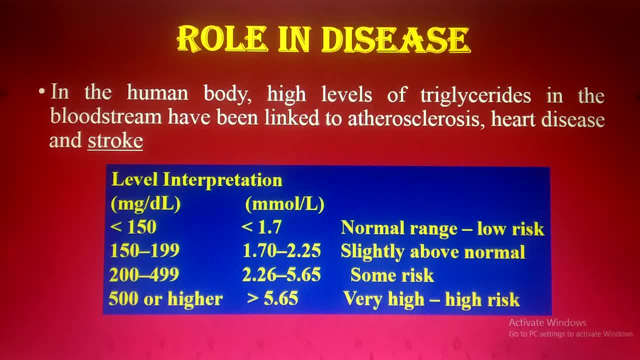 in the human body. high level of triglycerides in the bloodstream have been linked to atherosclerosis, heart diseases and strokes. so the level of normal level is less than 150 are in millimoles. you can see here less than 1.7 millimole per liter- milligrams per day in the blood stream. 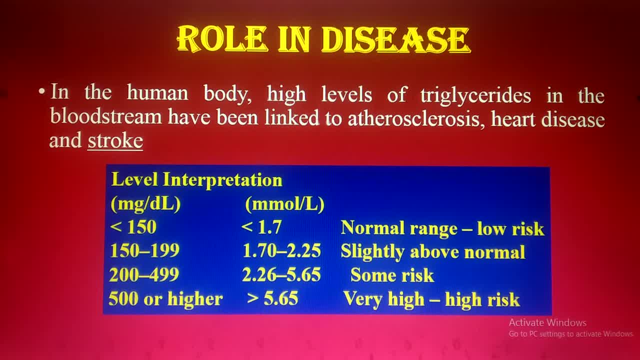 per deciliter: 150, less than 150, and millimoles. in millimole it is less than 1.7. this is the normal range, low risk. and 150 to 199. this is slightly above normal. 200 to 490- some risk. 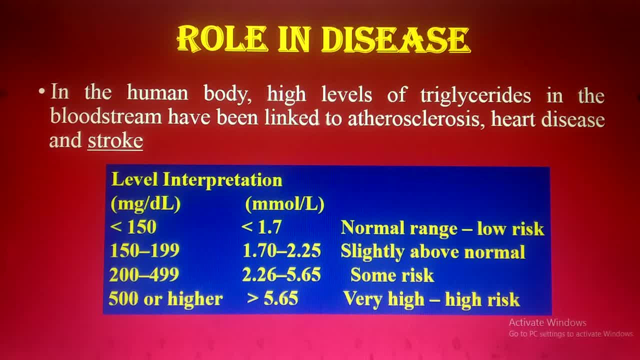 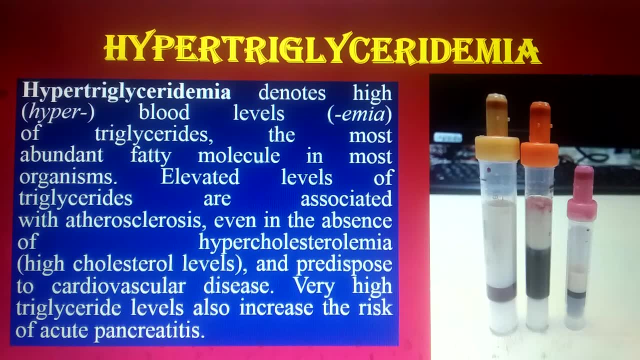 and 500 or higher. very high, high risk. okay, now there is a condition which is known as hypertriglyceridemia. now what is the hypertriglyceridemia? hypertriglyceridemia- the word hyper means high glyceryl, glycerdehyde, glycerides and imia means the blood. so the high level of the